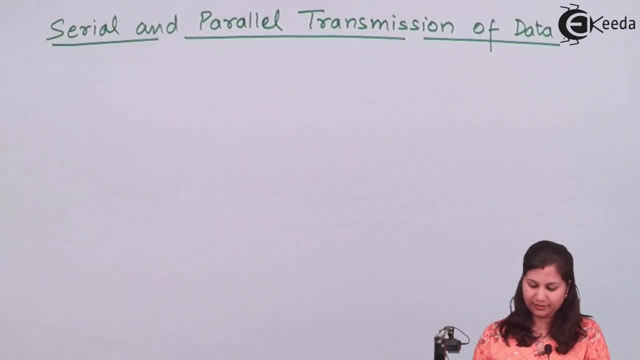 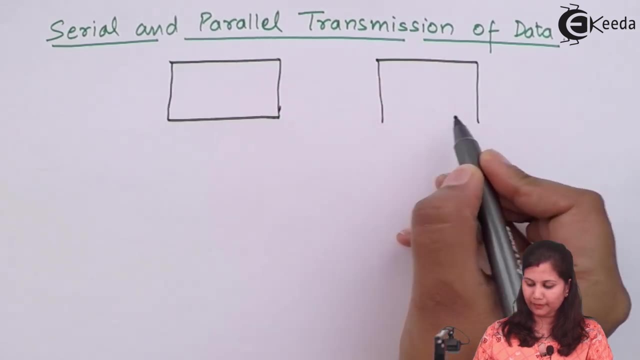 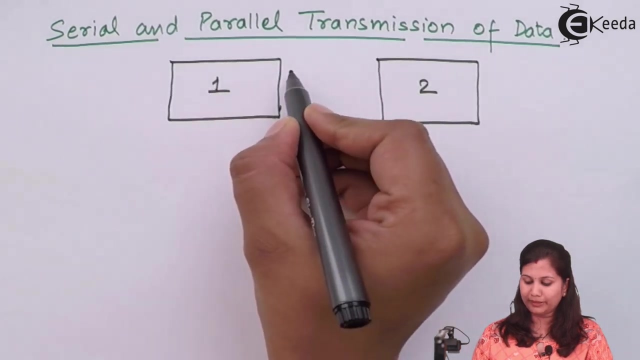 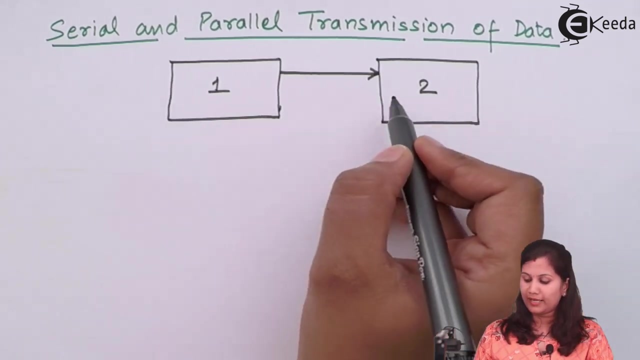 the data. So if we say that we are having two components and these components are communicating with each other, communication means that they are transmitting the data between each other. Suppose the component number one: it is sending the data. so component number two: it will receive that data. Suppose if component number 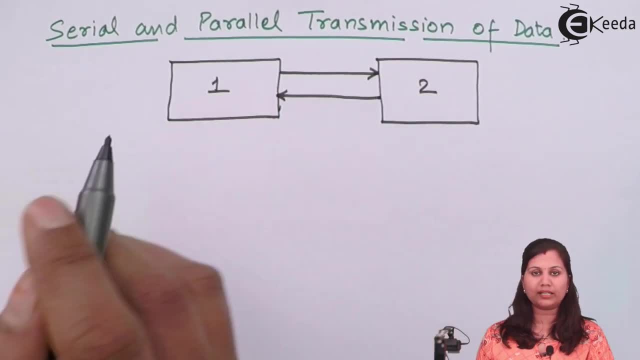 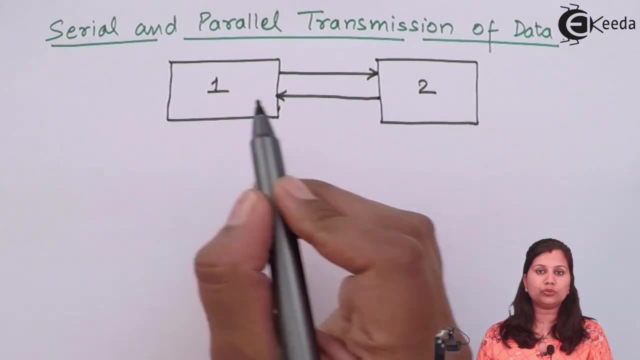 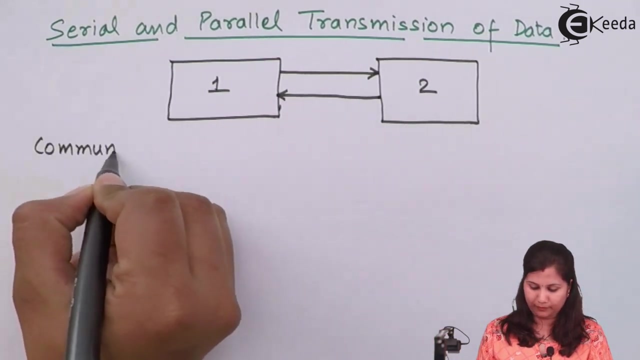 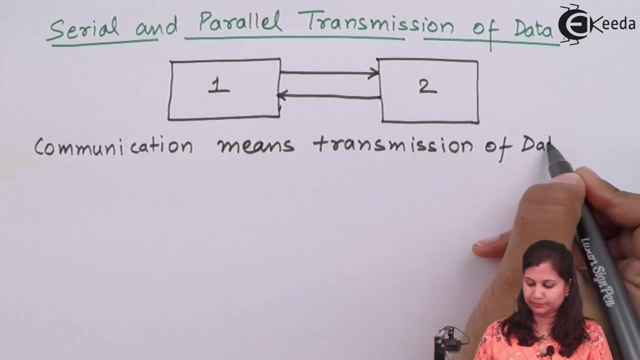 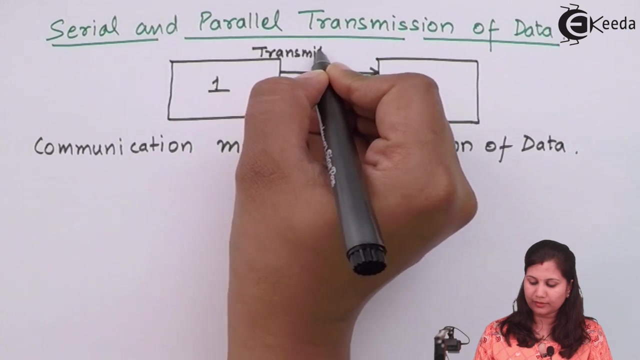 two, it is transmitting the data. and component number one: it is receiving the data. Means that transmission of data is taking place between the two components and that transmission of data is known as communication. Okay here, component number one: it is transmitting the data. component two: it is receiving. 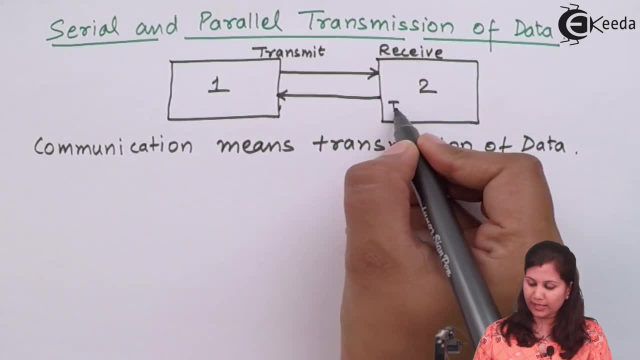 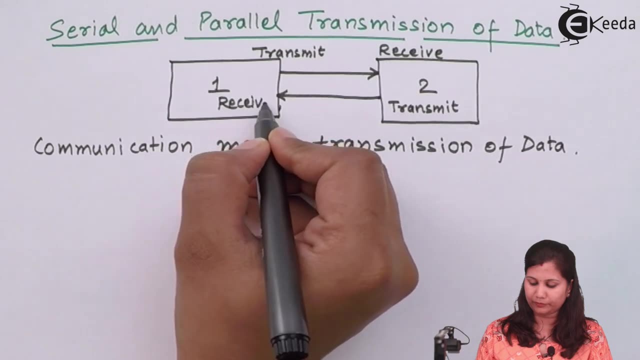 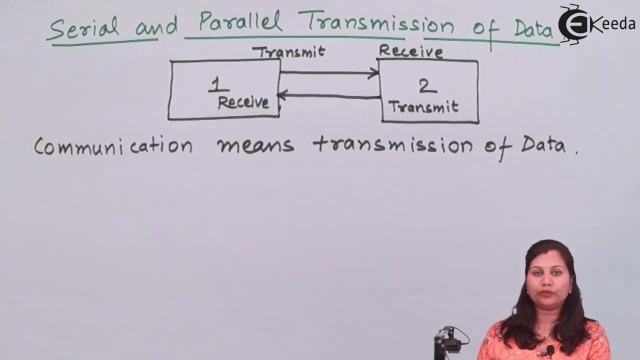 Here, component number two: it is transmitting, and component number one it is receiving. So data is being transferred between the two components. Now, this transfer of data, it can be of two types, either serial transmission or parallel transmission. So in this video, 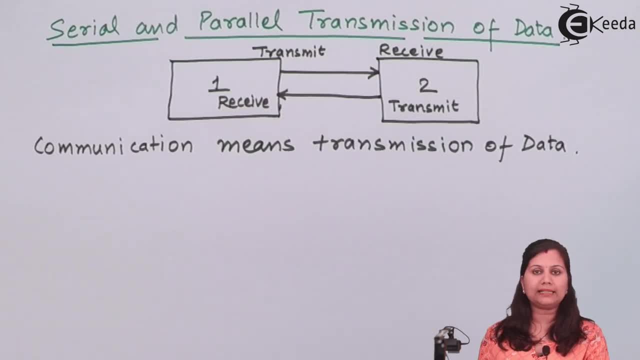 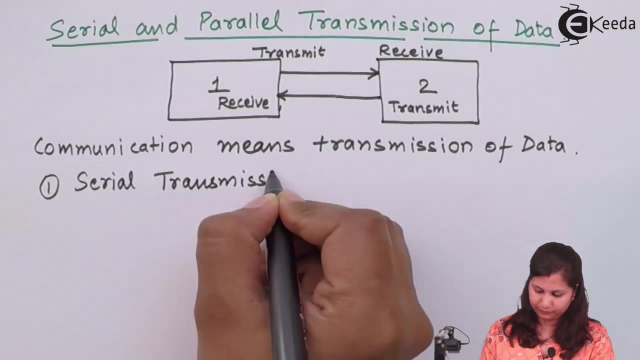 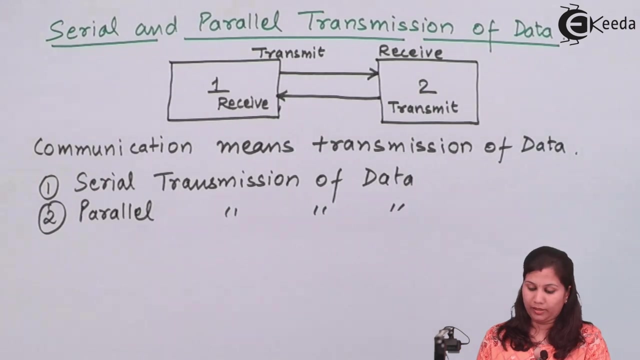 we will study that, what is called serial and parallel transmission of data. Okay, lets go back Now. if we take case of here, we are taking component one and component two. if we take case of computers and microprocessor which deals with the data which is in the form, 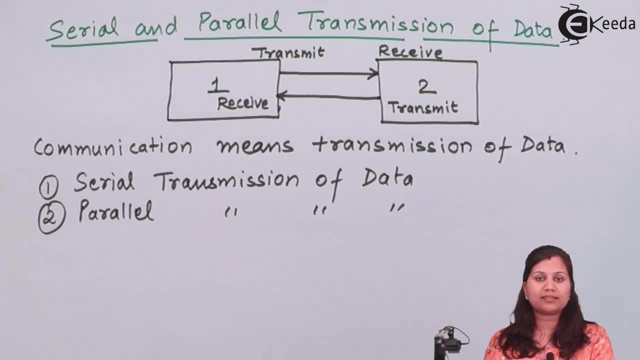 of bits. so when data is transmitted, it means the bits of that data are being processed and earraped, transmitted. now, in case of serial transmission of data, only one bit is transmitted at a time, okay, and in case of parallel transmission, all the bits. 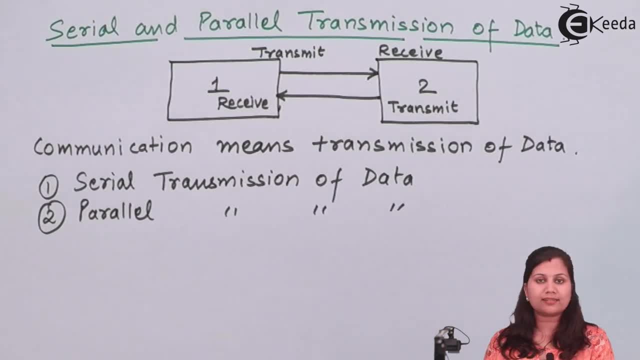 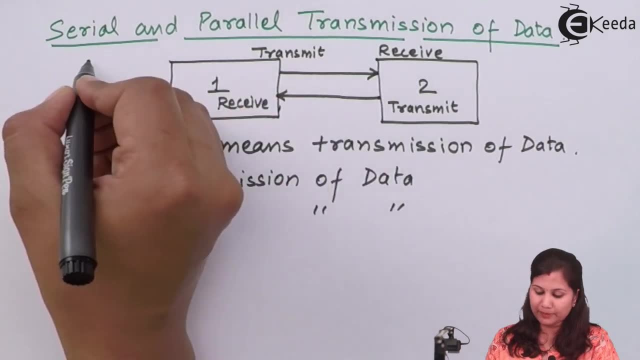 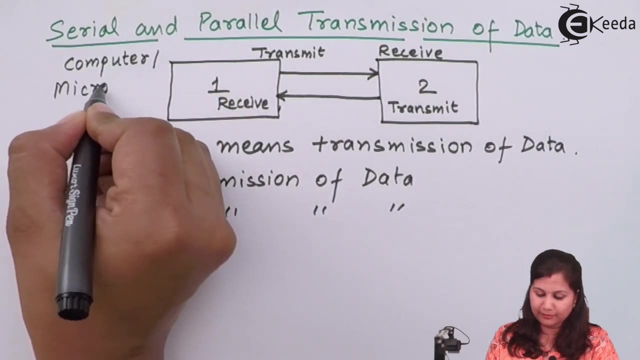 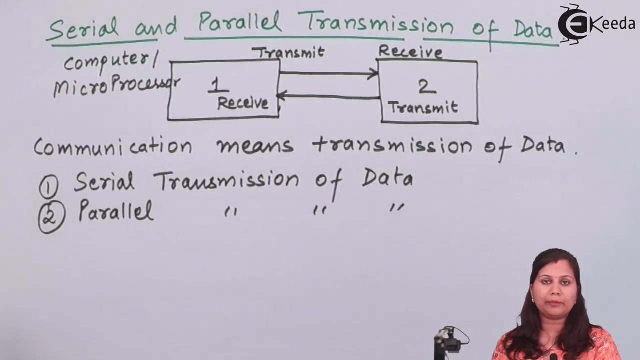 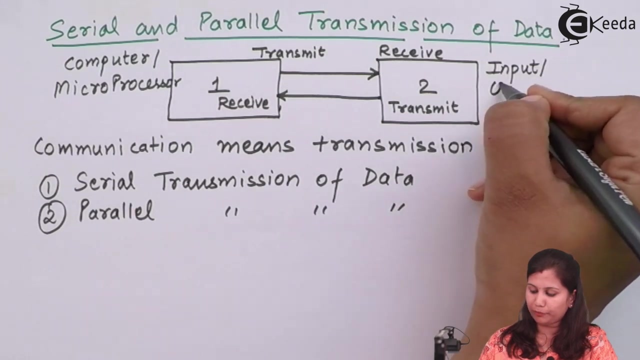 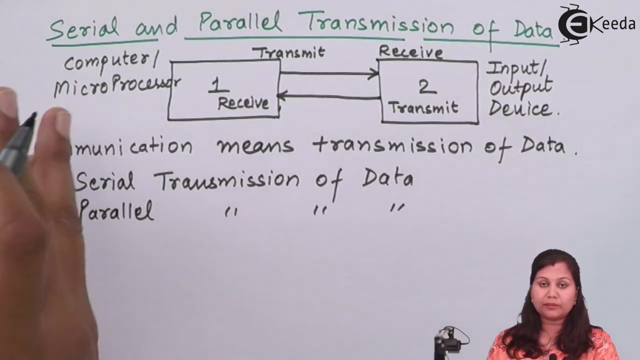 are simultaneously transmitted. so that is the difference between serial and parallel transmission of data. so in that case, component one, it becomes either a computer or it can be a microprocessor. okay, it means any kind of programmable component can be there, and at the end here we can have any input or output device. so whenever computer or 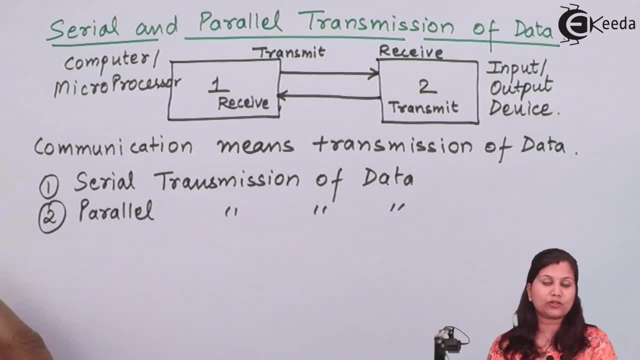 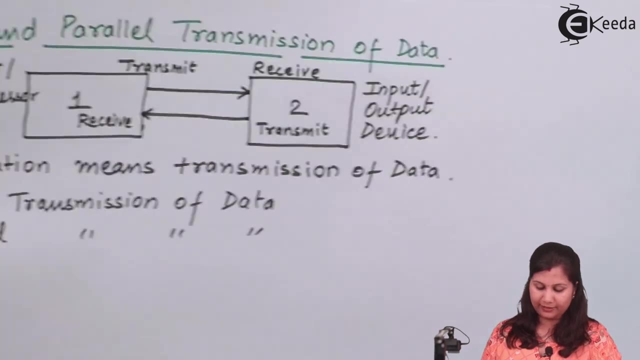 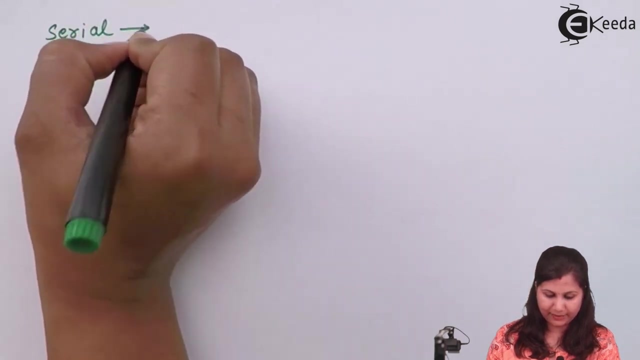 microprocessors. they are communicating with each other with the input output devices, or we can say the peripheral devices, so they either they can use the serial transmission of data or they can use parallel transmission of data. so let's see the difference in serial transmission. as I have said that one bit. 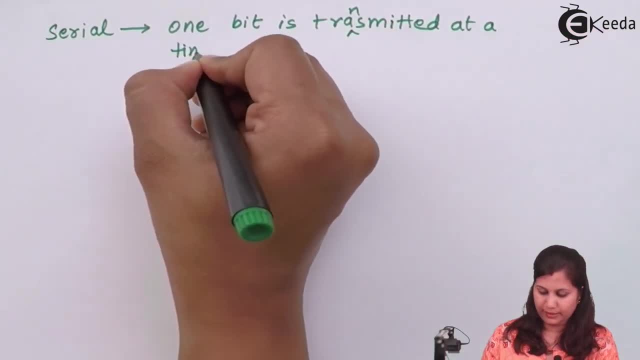 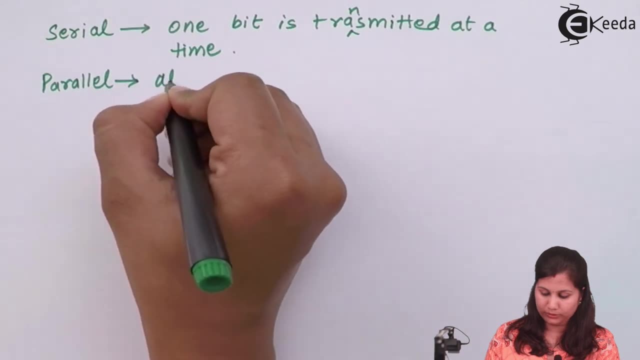 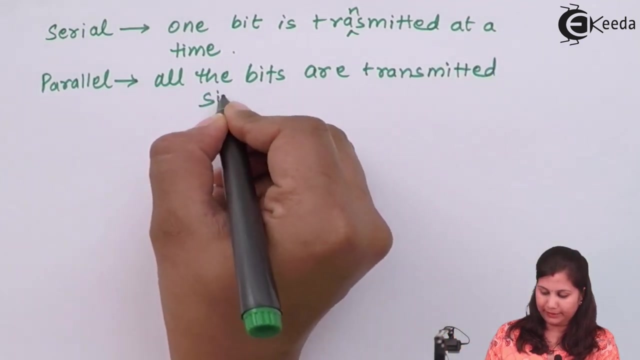 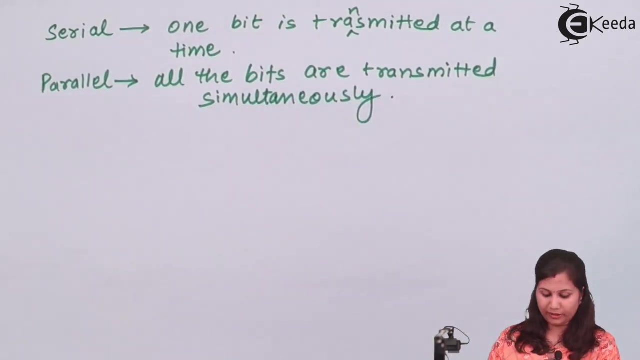 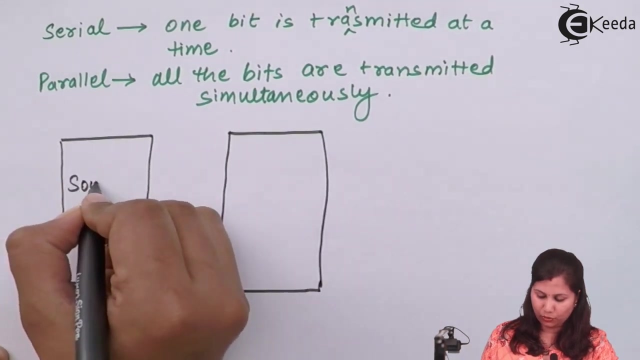 is transmitted at a time, whereas in parallel all the bits simultaneously. now, if we describe it in the form of a diagram, then the Suppose it is the source and it is the destination Source is sending the data to the destination in the using this serial transmission. 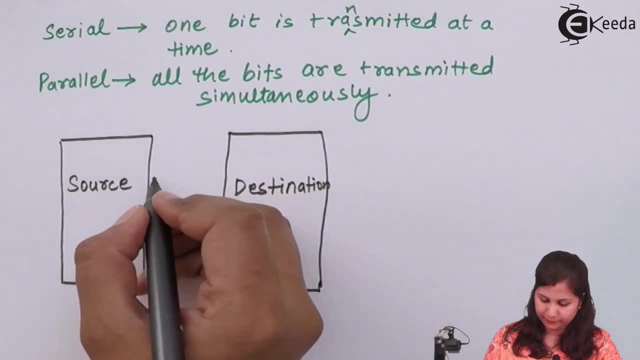 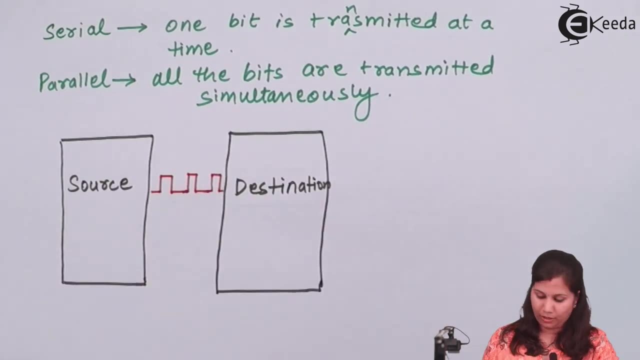 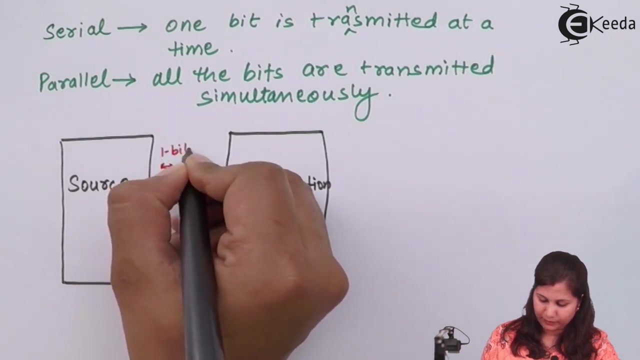 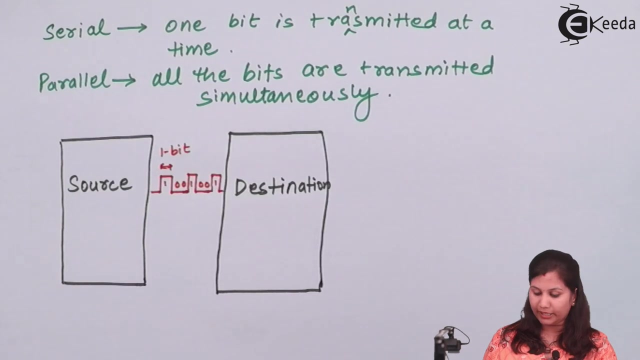 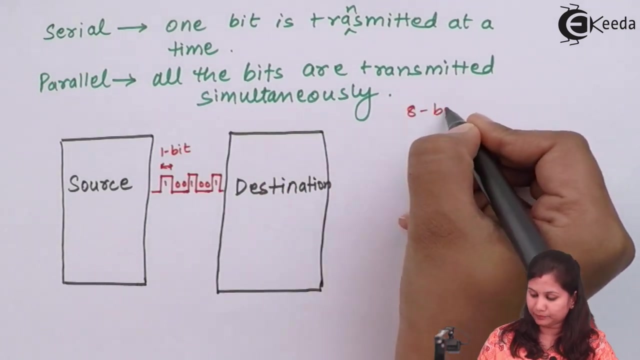 So in serial transmission only one bit is transmitted. So suppose here one bit is transmitted. This is one, this is zero. again, zero one, zero, zero one. okay, In the form of this data is transmitted. Suppose we are having a data, 8 bit data, is there one zero, zero one, one zero zero. 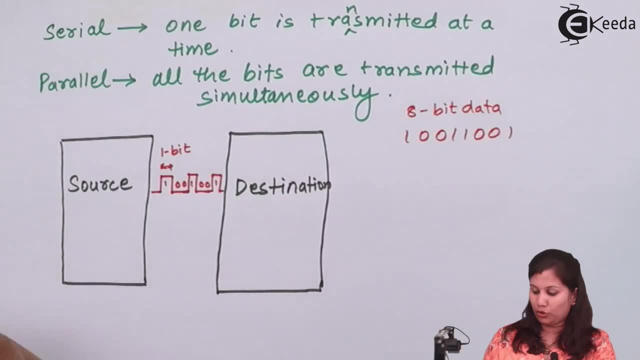 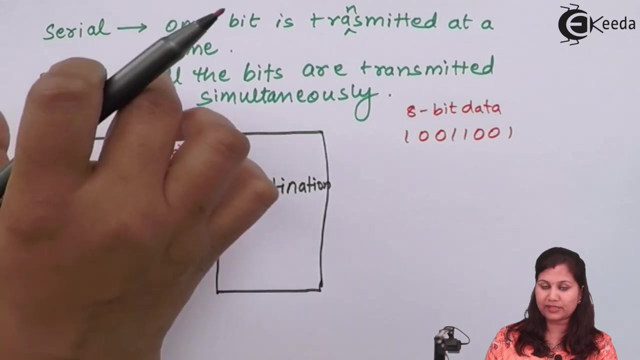 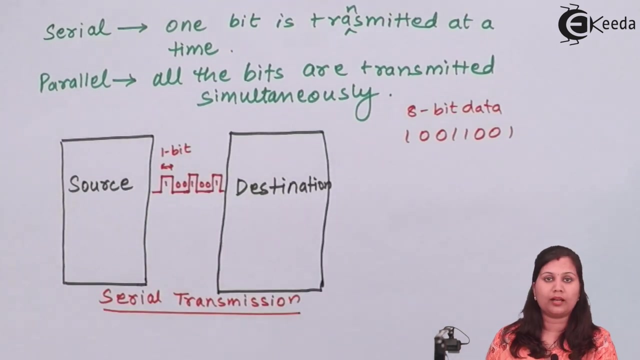 zero, one. So if this data is to be transmitted, first one will be transmitted, then zero, then zero, then one one, zero, zero one. So in this form data is transmitted in the case of serial transmission, But in the case of parallel transmission, all the 8 bits, they will be simultaneously. 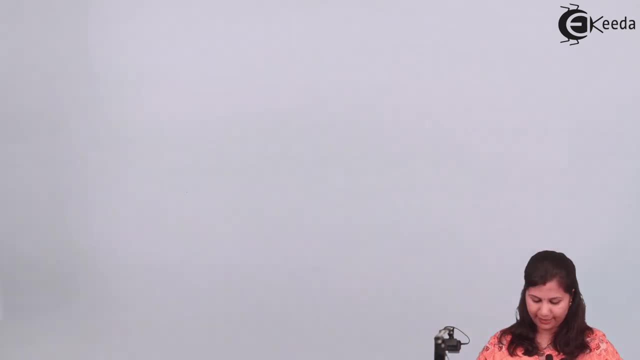 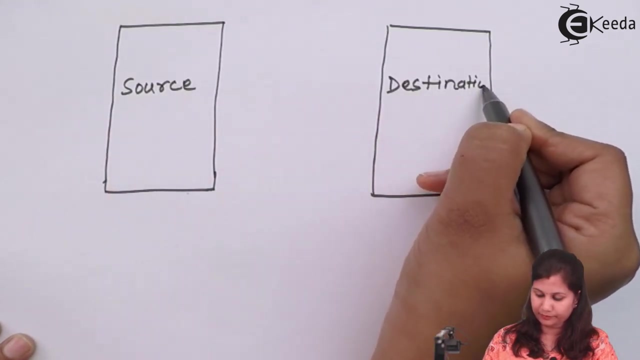 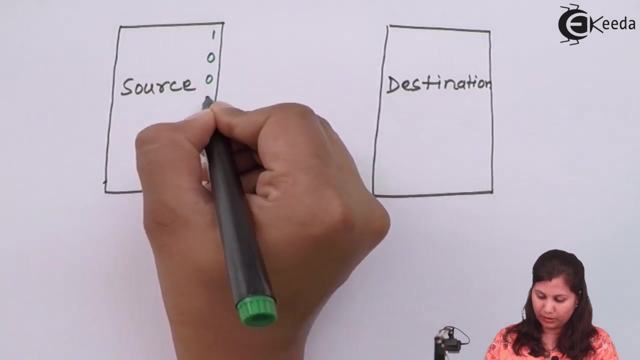 transmitted. So if we denote it by the diagram we will have, Suppose this is the source, it is the destination. We were having the data: one zero zero one, one zero zero one. So first bit is transmitted. 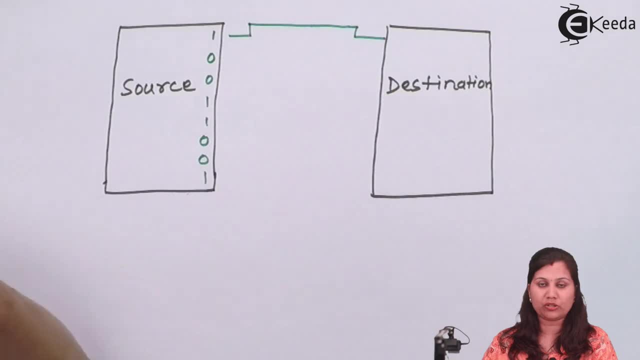 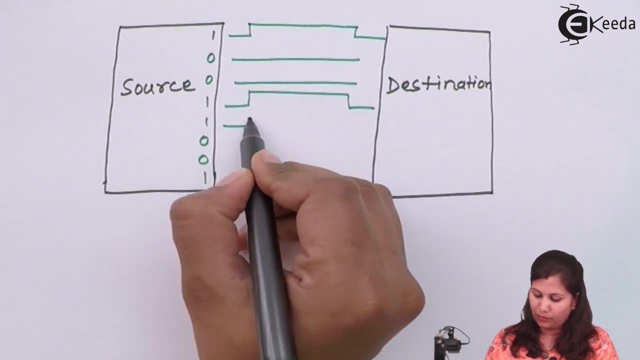 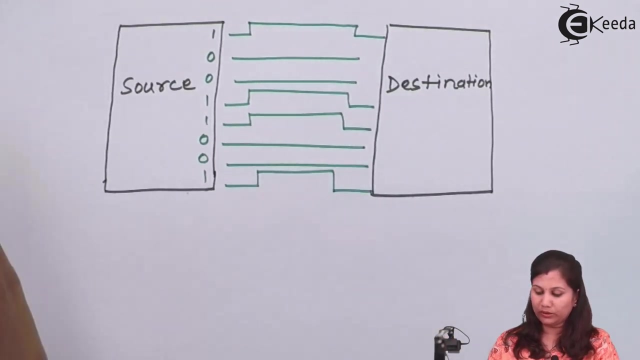 One, so one will be transmitted. second is zero. zero is transmitted, again zero, again one. one zero, zero and again one. So in this way all the 8 bits are simultaneously transmitted, and that is the case of parallel. 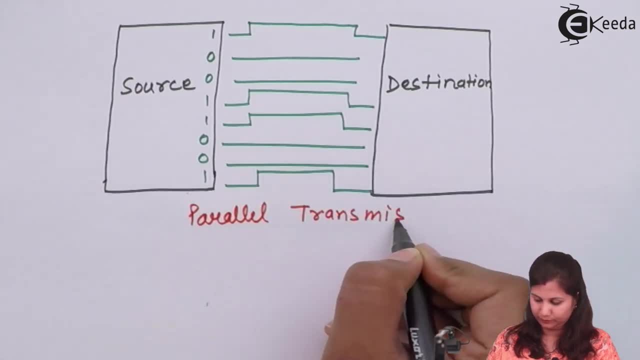 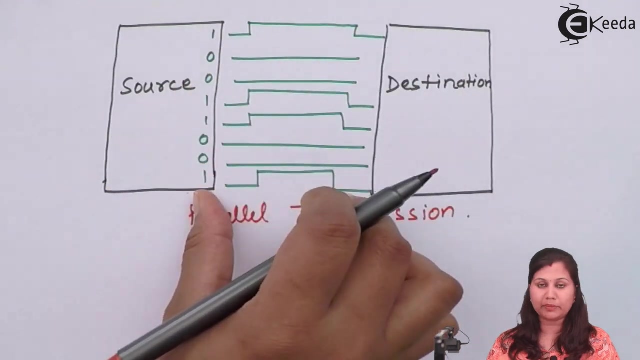 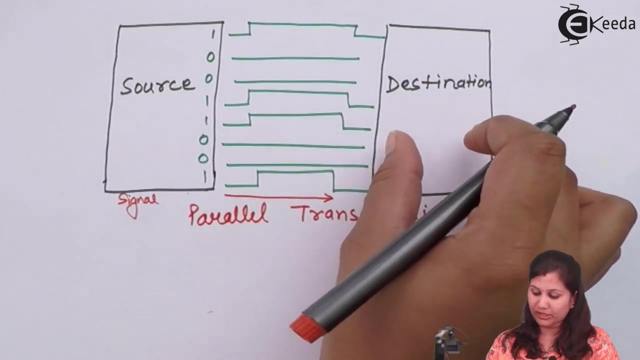 transmission In the case of transmission, Okay, Okay, Okay. So in parallel transmission, along with the data which is transmitted, a signal reference is also transmitted. So here, along with these 8 bits, a signal reference is also transmitted, So that the destination, the component which is there, it can compare the data received. 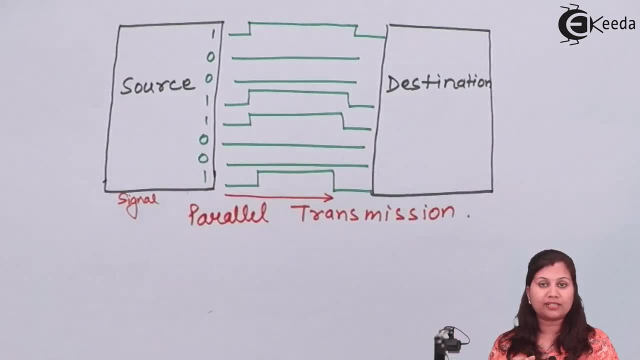 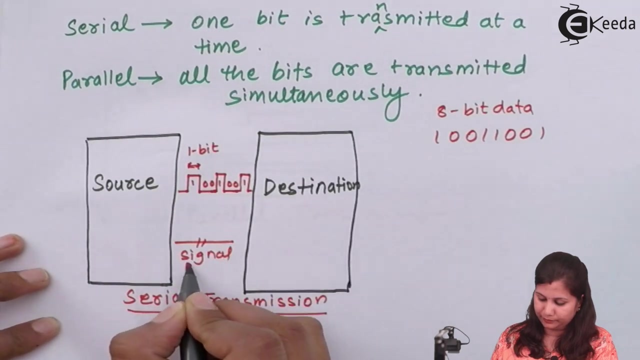 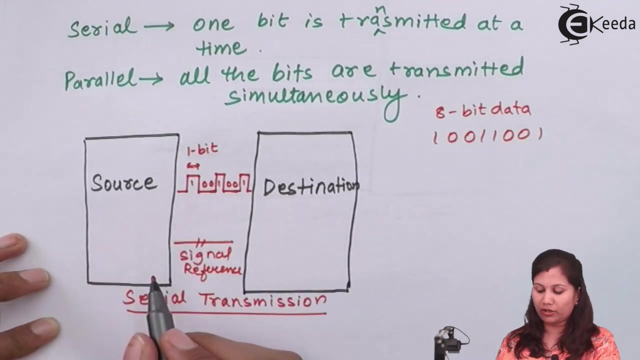 with this signal reference that the data which is received, that is correct or not. Okay, Okay, Okay, Okay, Okay, Okay. In case of serial transmission also, we have a signal reference here to check that, whether the received data and the actual data, they are equal or not, correct data is received. 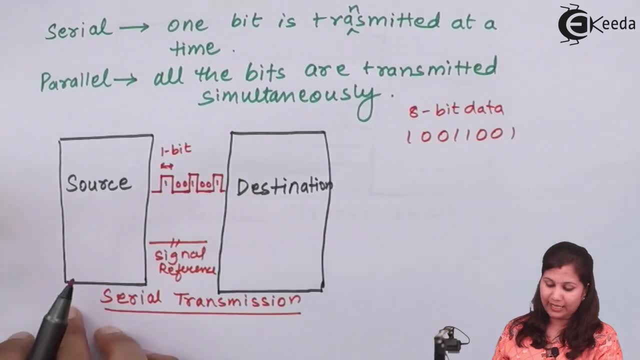 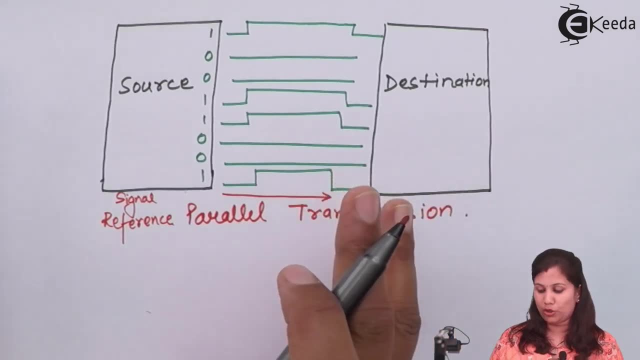 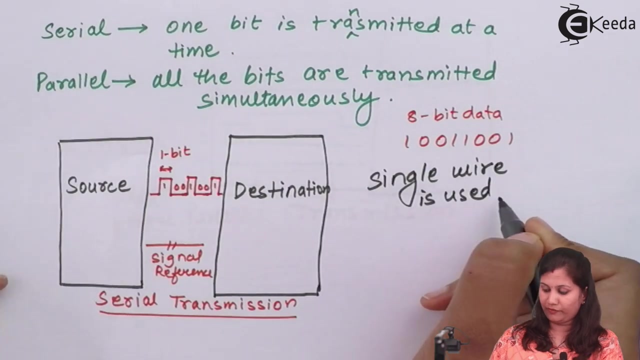 or not, by the destination. So you have seen that in serial one bit is transmitted and in parallel all bits are transmitted simultaneously. see this? the difference come that in case of serial transmission, only single line is used, single wire is used to transmit the data, whereas here, if we want to transmit 8 bits, 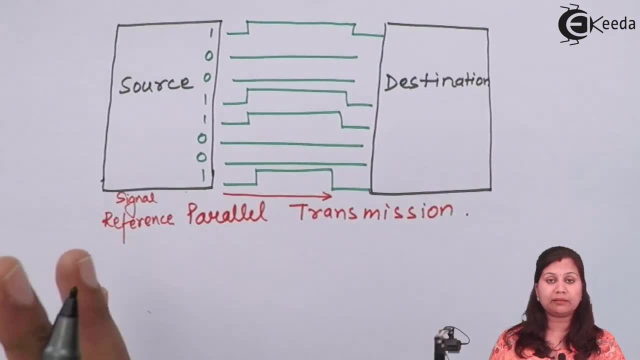 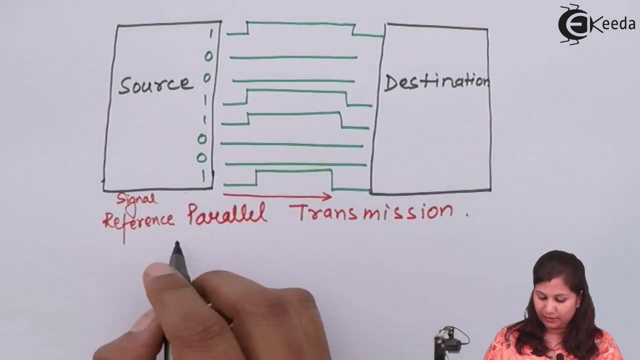 so we have to use 8 lines. if we are transmitting 16 bit data, then we have to use 16 lines. if transmitting 32 bit data, then we have to use 32 lines. so according to the data, the lines which are used to transmit the data, they are increased. so here many wires or lines are used. 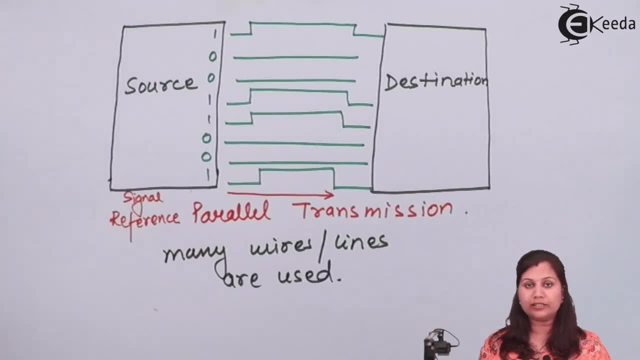 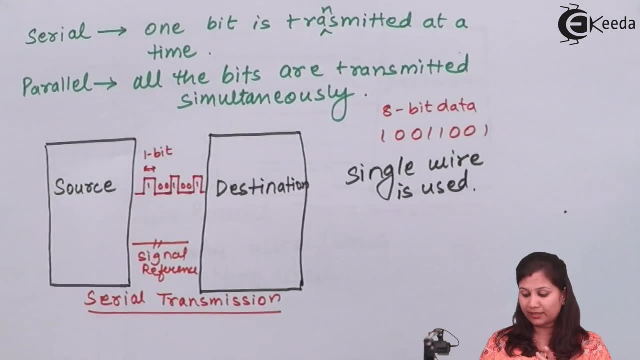 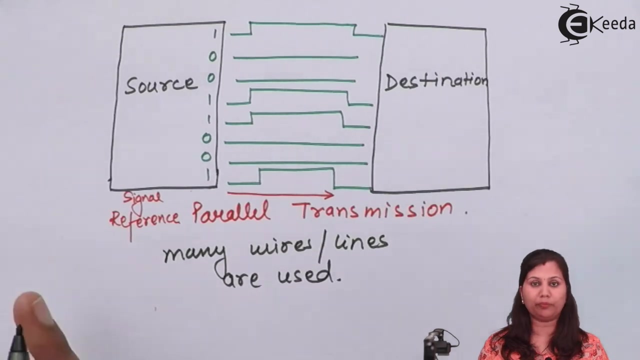 so that is one difference- that in serial transmission only single wire is used. so here less circuits are used. less means the circuitry for the serial transmission is less bulky, whereas in the case of parallel transmission it is more bulky because for separate bits we have separate wires, each bit is acquiring separate wires. now here, because if we are 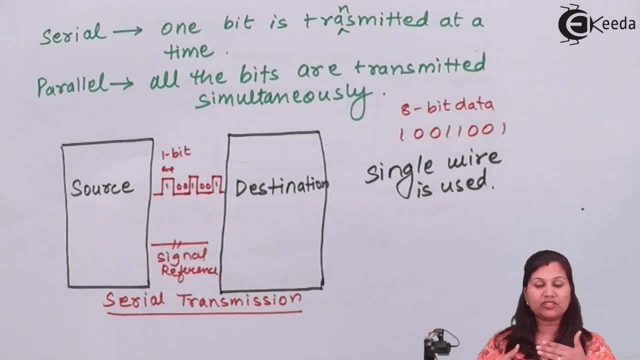 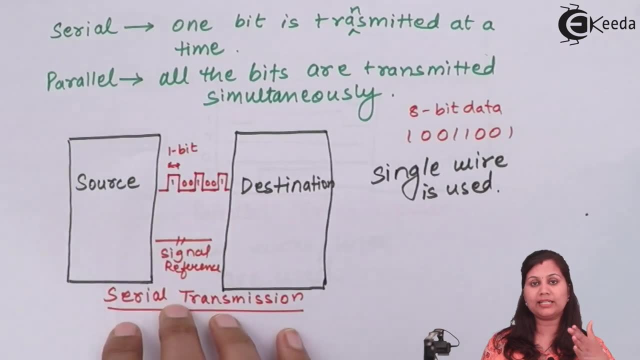 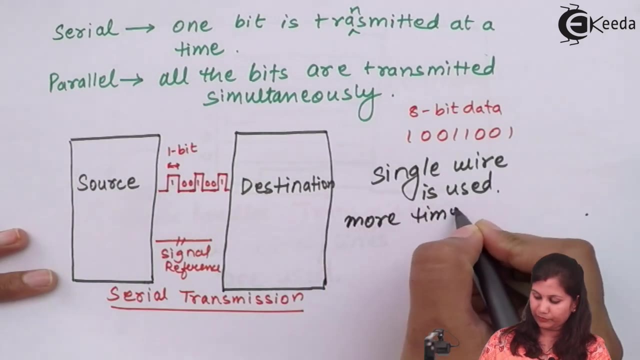 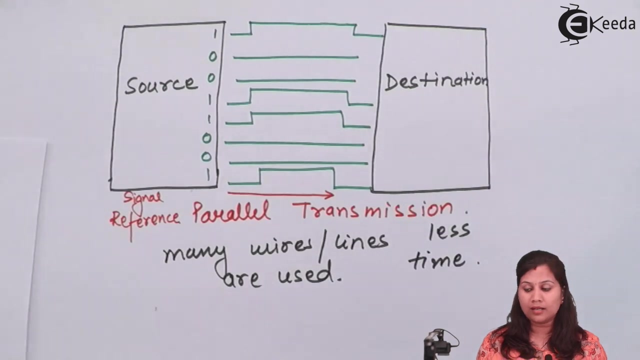 transmitting 8 bits it will take a long time because only one bit is transmitted at a time, whereas in case of parallel because all bits are simultaneously transmitting, so it will take less time. so here will have more time required of parallel. less time now as time is taken less in parallel transmission and 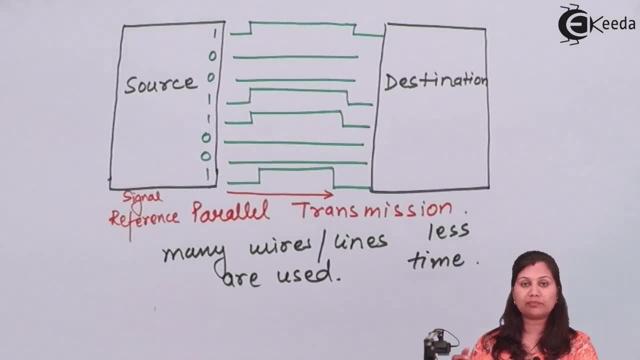 more time is taken, but whenever we want to transmit the data over long distances, it is very difficult to use the parallel transmission because for long distances we cannot use so many wires because each bit is having a separate wire. so if we want to transmit 16-bit data we have to join 16 lines between the input output. 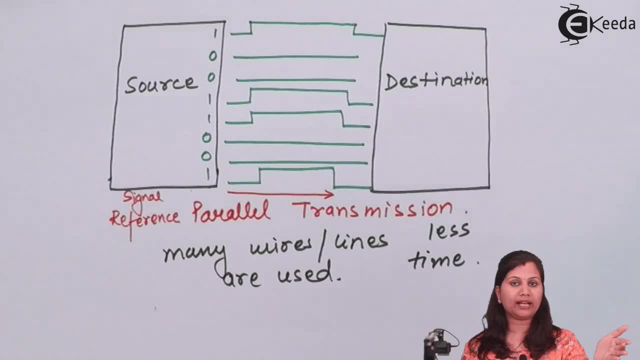 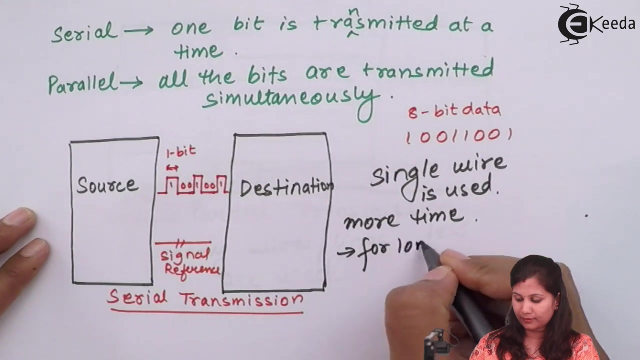 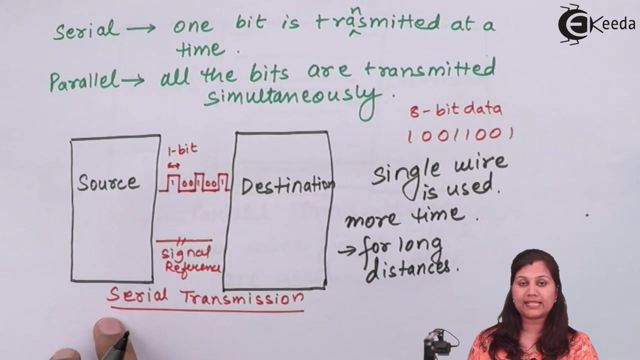 devices and the suppose computer and microprocessor we are using, so so many wires we have to use, and those wires cannot be used for long distances. so for long distances we prefer serial transmission over parallel transmission. so we can say that for long distances serial transmission is used, but for short distances parallel transmission is. used because parallel transmission is faster than serial transmission. here one bit. so if we are transmitting 16 bit of data so it will take a long time to transmit the data, whereas if we are using parallel transmission all 16 bits are transferred simultaneously. so for short distances we will prefer. 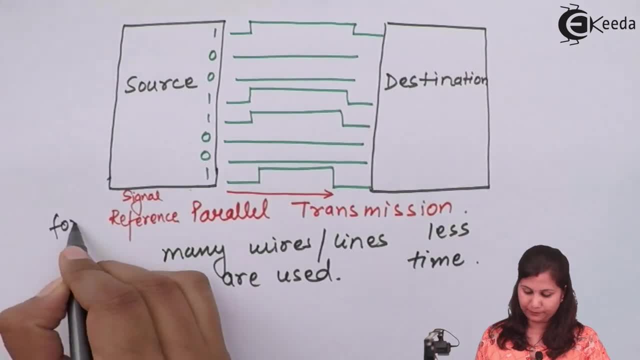 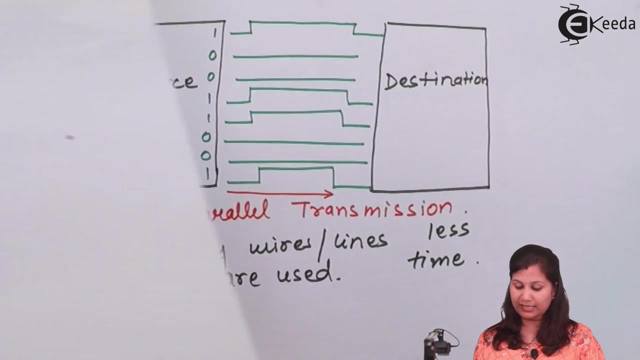 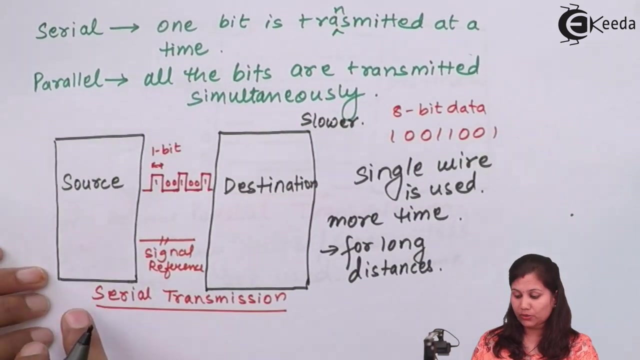 parallel transmission also. this parallel transmission is taking less time, so it will be faster, whereas serial transmission it will be slower. ok also this serial transmission, because it is using single wire, less hardware circuit is required, less cable cost is there, so we can say that they are less, so they. 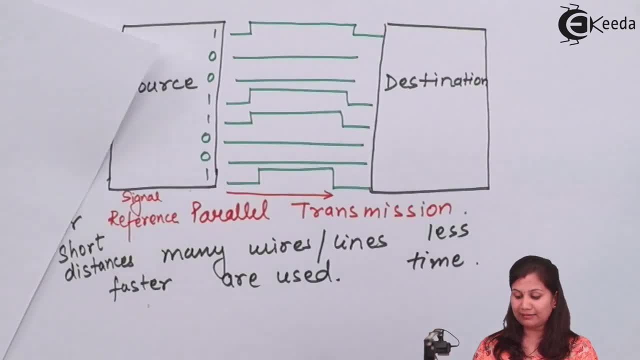 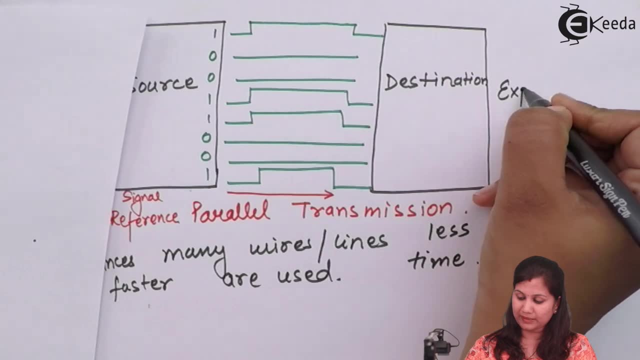 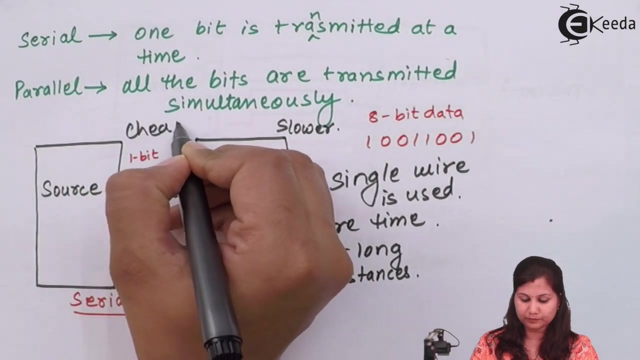 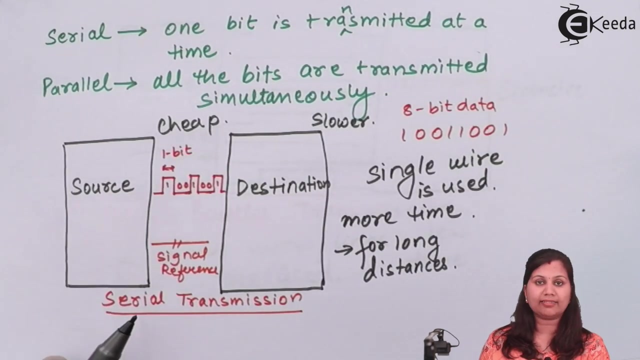 are taking less cost, they are cheap, whereas the parallel transmission it is very expensive. ok, because so many wires are there, so we can say that it is expensive, whereas serial transmission it is cheap. so these are some of the features of serial transmission, which means you have to ultimately transmit legal data for long distances. 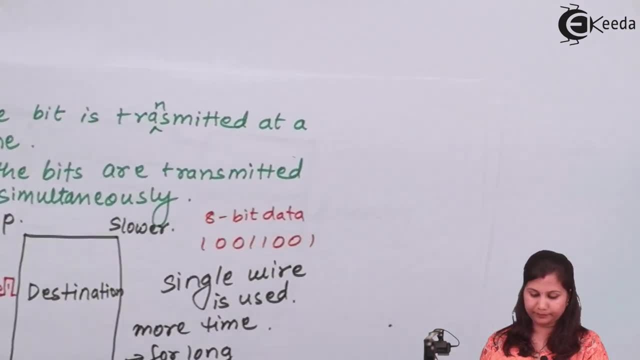 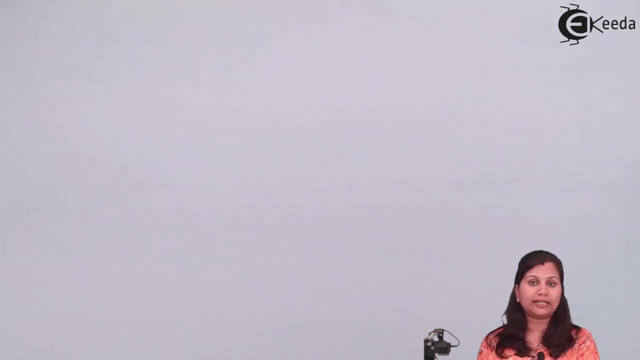 so for the work of serial transmission is very important. so these are the parameters. sol properties for becomes the intervention we will talk about in a little bit further. let me give you some data on these 蝏 n SSC, what you are doing now. 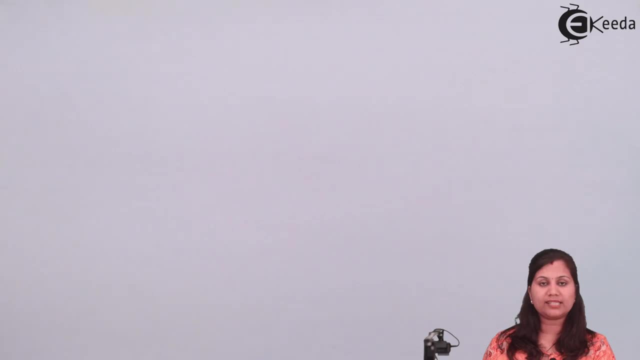 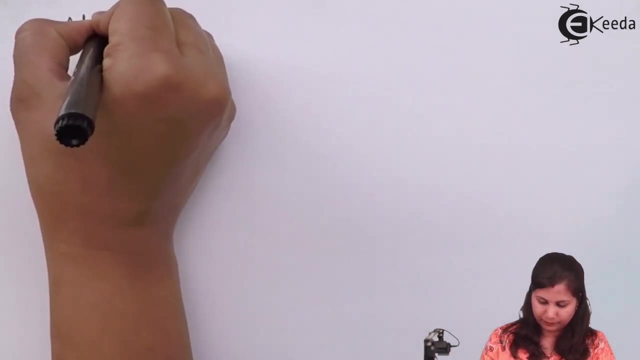 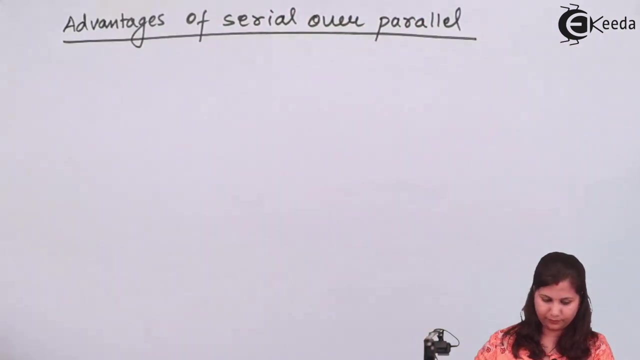 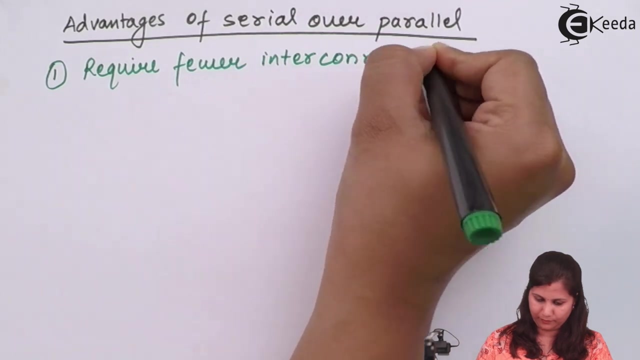 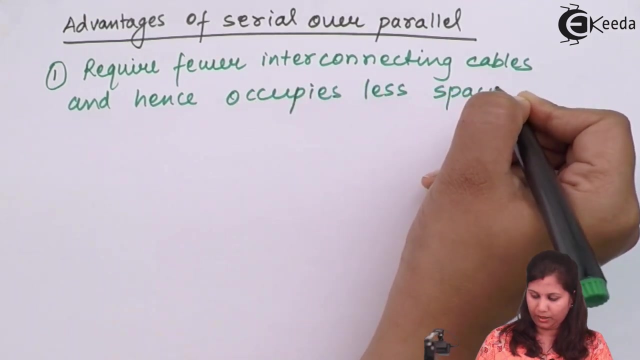 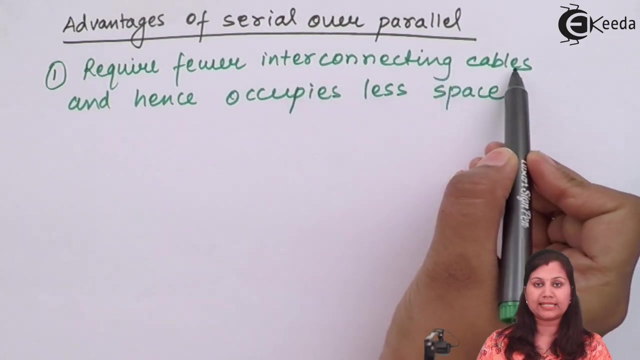 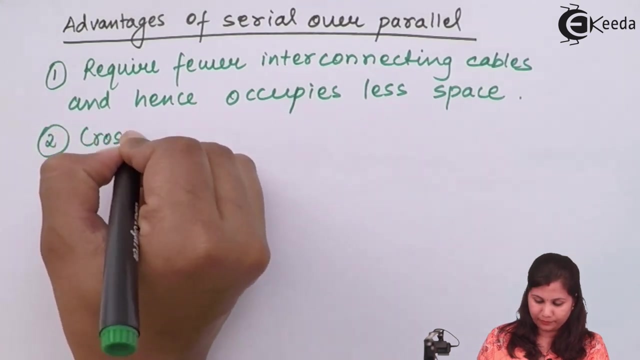 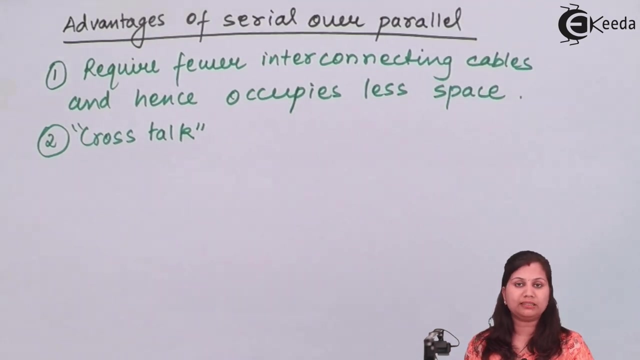 advantages. So let's see that. what are the advantages? why serial transmission is preferred over parallel transmission? The serial transmission because only single line is used, so it requires fewer interconnecting cables and hence it occupies less space in comparison to parallel Cross-talk. it is a kind of problem which occurs whenever we are transmitting the data Cross-talk. 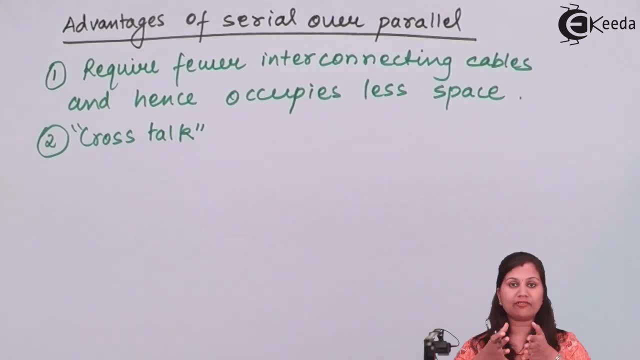 means that when we are using several wires, then the data which is transmitted at each wire, It can be mixed. okay, so that case is not in the case of serial transmission, because there is only a single line over which we are transmitting all the data, so there is no cross-talk issue. 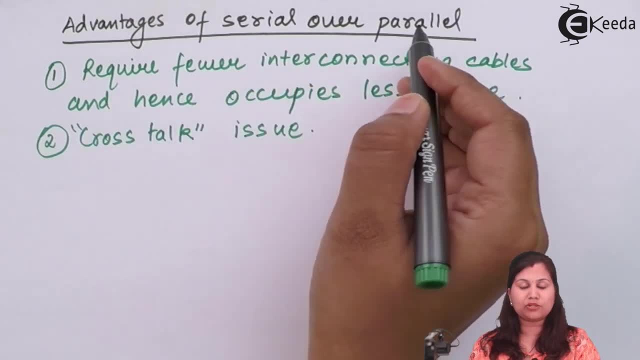 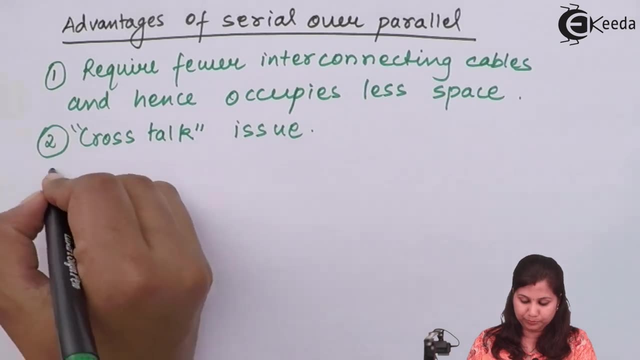 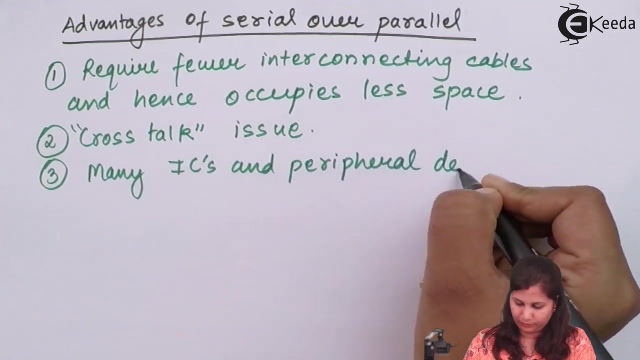 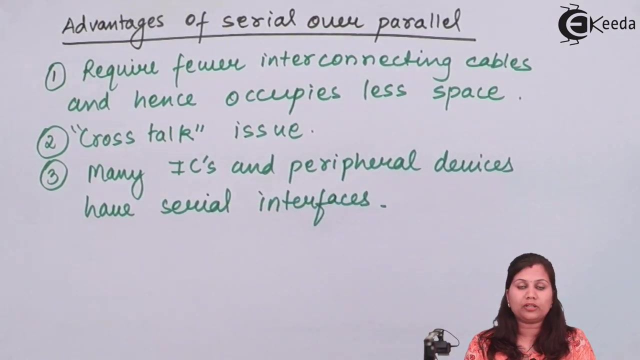 in the case of serial transmission, whereas in parallel transmission, because there are several wires, so the wires data, they can be mixed. cross-talk issue can occur, Now that we know that the signal is transmitted through the microprocessor. it also has a common side, as we know that the signal is transmitted through the microprocessor, but 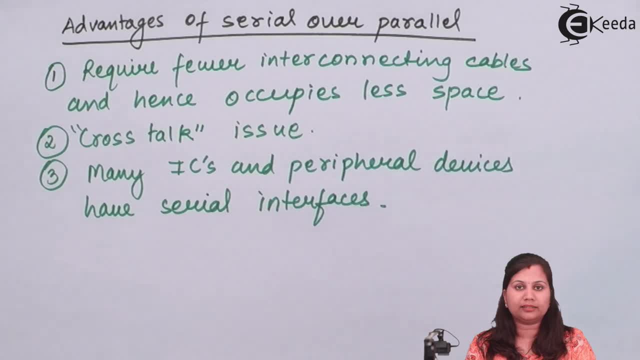 the signal is transmitted through the receiver and the server and the receiver can also be transmitted through the receiver. Now let's see that. what are the disadvantages of that? Let's see the most important one: why computers and microprocessors have to use serial transmission of data Parallel. 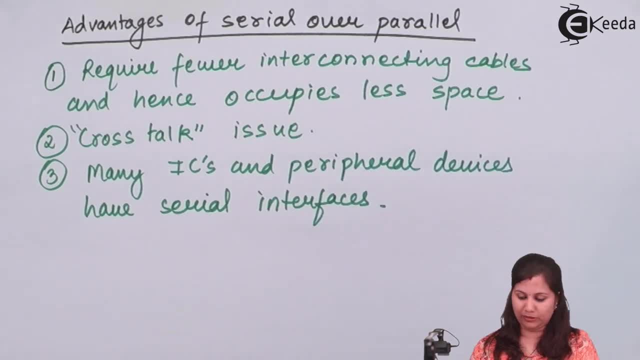 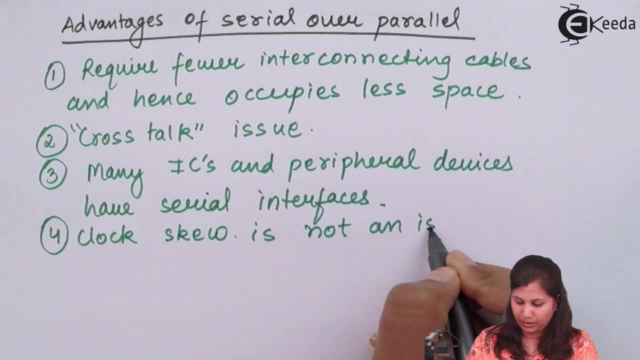 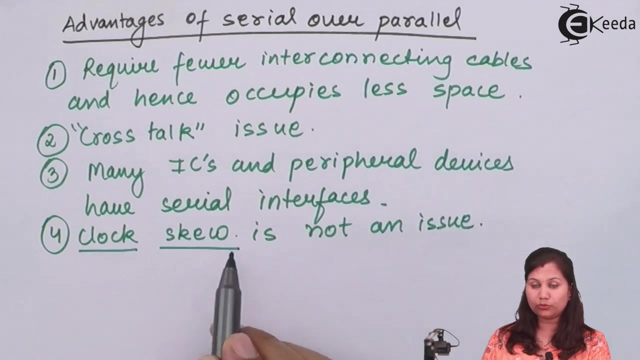 data has to be converted into serial data for the transmission. Another problem which occurs in the case of transmission of data: it means that is called the clock skew. Clock skew- it is a kind of phenomena which occurs that suppose in computers we have different blocks and each block want the clock signal. Now, when the clock signal